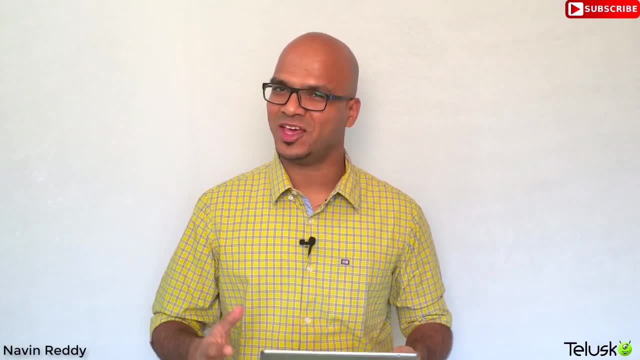 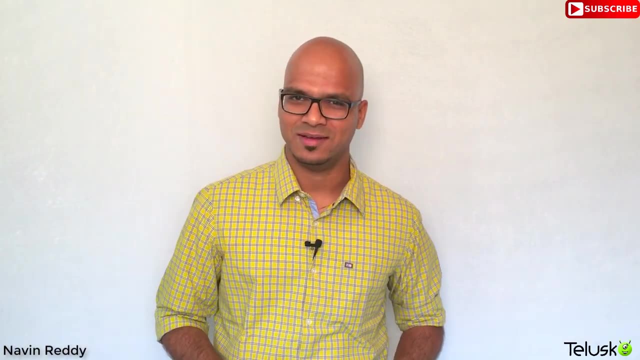 So what you think. How many programming languages are there in the world? Maybe 5, 10,, maybe 50,, maybe 100,, maybe 1000?? Make a guess And the answer is there are more than 10,000 languages available in the market. 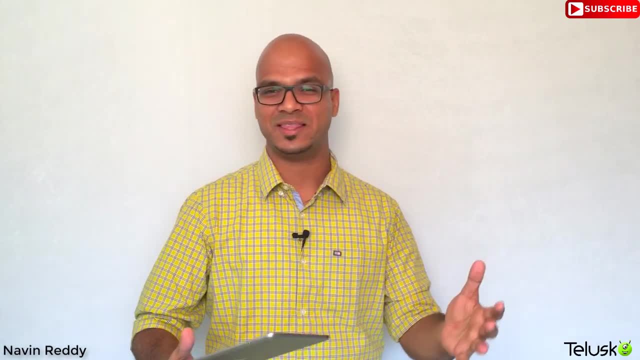 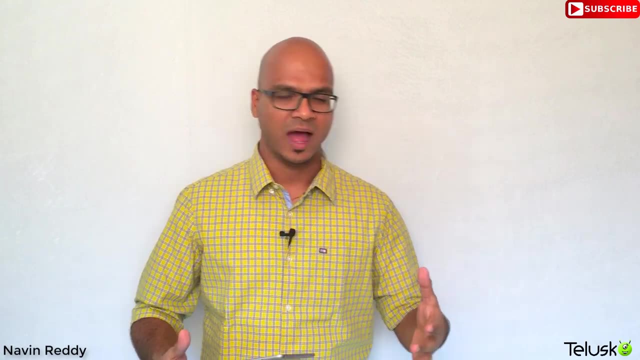 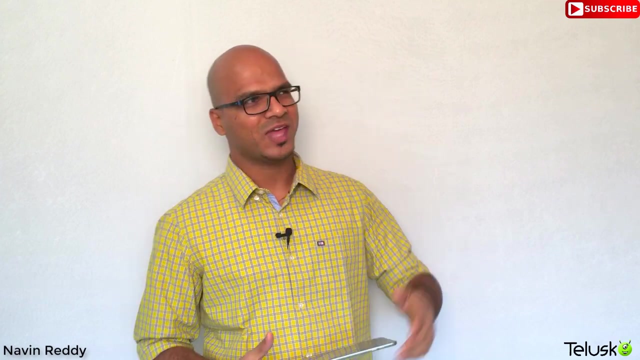 I mean, think about this. Why would anyone would create 10,000 languages, right? It's because there is not one person who is making all these languages right. There are different people working on these programming languages. In fact, I feel you know, if you are working on- I mean, if you are doing your PhD, if you are doing some research- and you will be thinking, you know we have lots of programming languages. Can we create our own language which will be better than this? 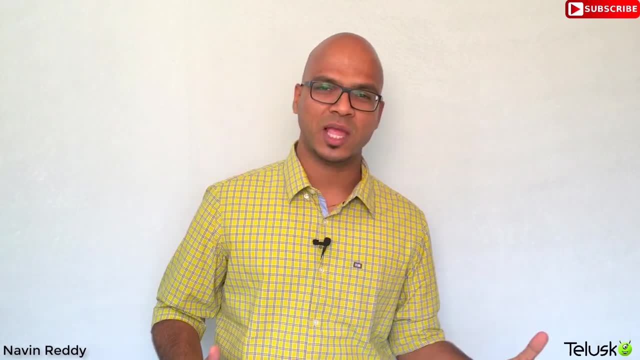 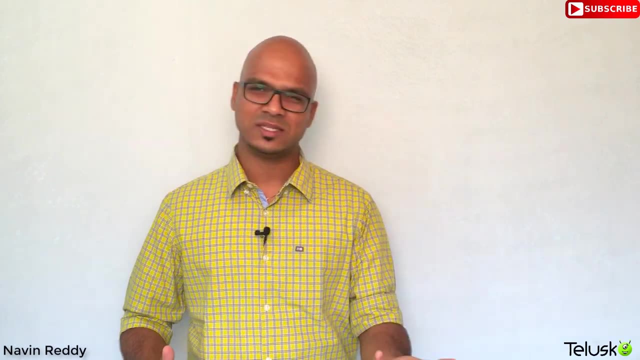 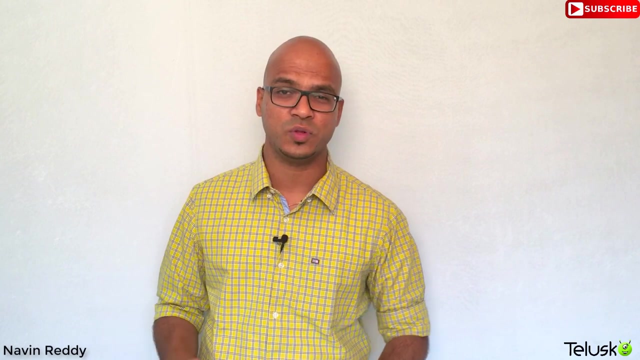 In fact, sometimes I feel that C programming is best, Sometimes I feel PHP is good, Sometimes I feel Java is best. And then, you know, I think, can we just merge all these concepts and then come up with a new language? And that's why we are getting new languages every year or every two years? 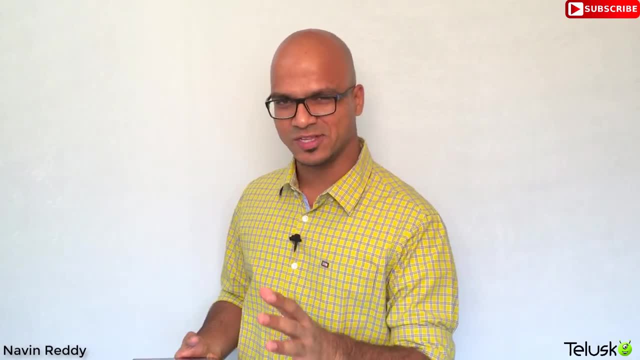 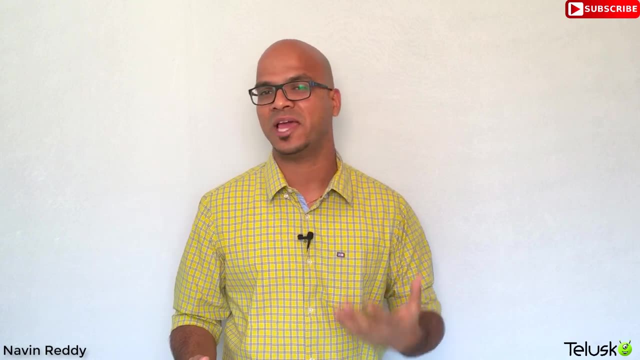 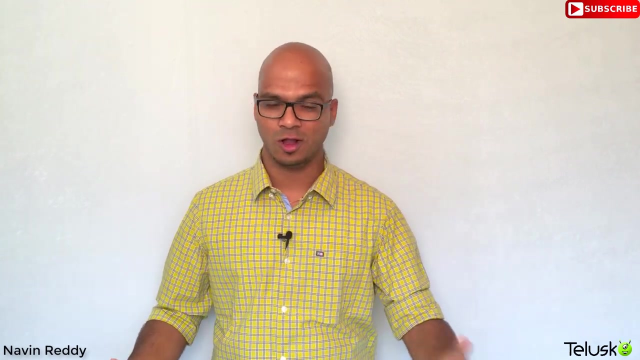 So there are approximately 10,000 languages and how many we know. maybe we heard about maybe 20, 30- and how many we know as a programming language, maybe one or two, right? So in this video we will talk about the series of programming languages- not all, not 10,000- but then we will talk about the series of programming languages which starts from 1843. 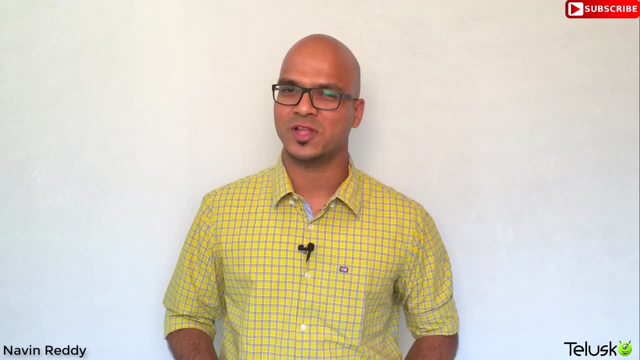 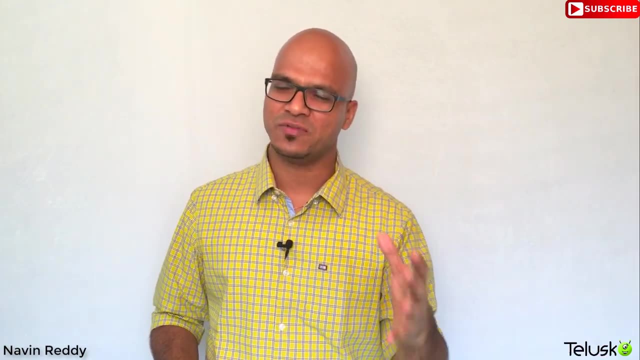 So welcome back aliens. I am Navin Reddy from Third School Learnings and in this video we will talk about history of programming languages. So let's start with the first programming language. I mean, can you guess in which year we got a programming language? Maybe 1990s? No, because C came before that. Maybe 1960s? No, because there were languages before that as well. What if I say the first programming language came in 19th century? I know you will not believe that, because the first computer itself came in 20th century, right? 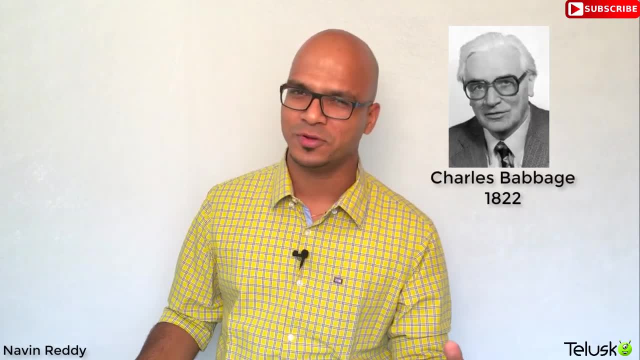 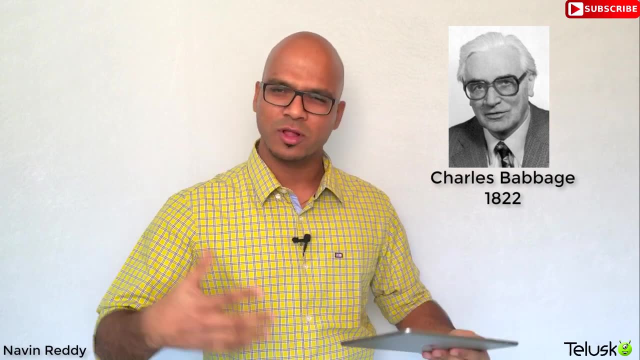 So what happened? you know, You heard about Charles Babbage right, The father of computer, In 1822, when Charles Babbage was working on the mechanical computer, and so he thought about a concept where you can actually implement a computer. 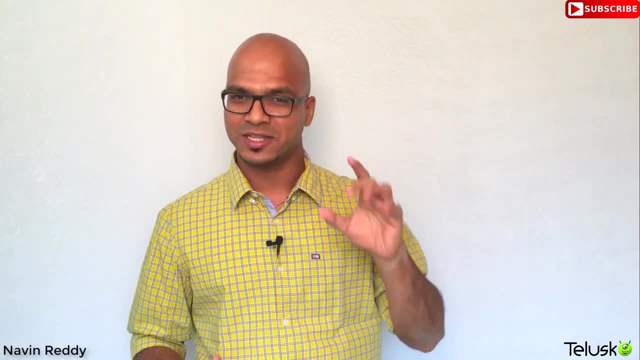 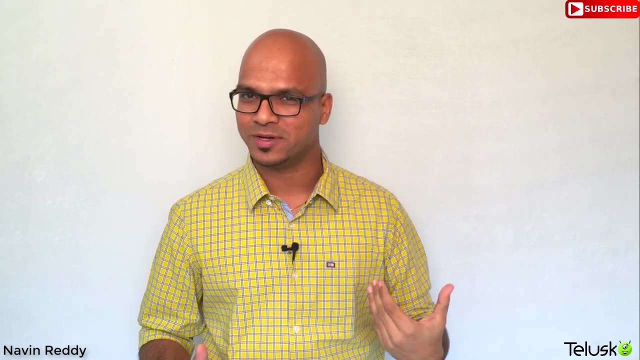 In fact, before that, in 16th century, there was a term called as computer Person who calculates. you know, as a person, if I use a calculator, I will be called as a computer, and that will be awesome, right, Calling humans as computers. 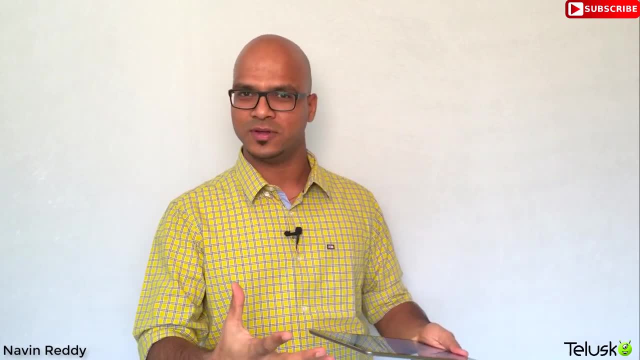 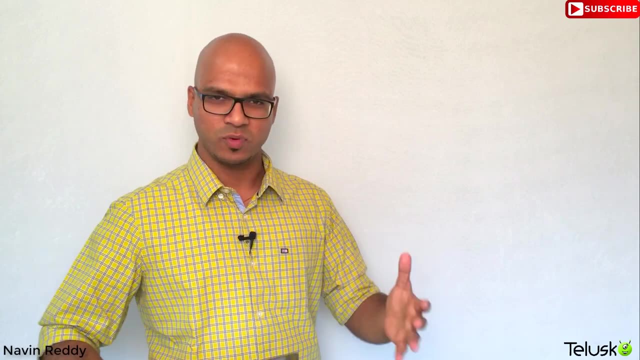 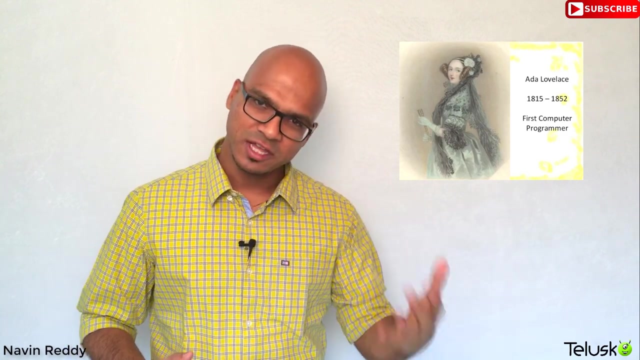 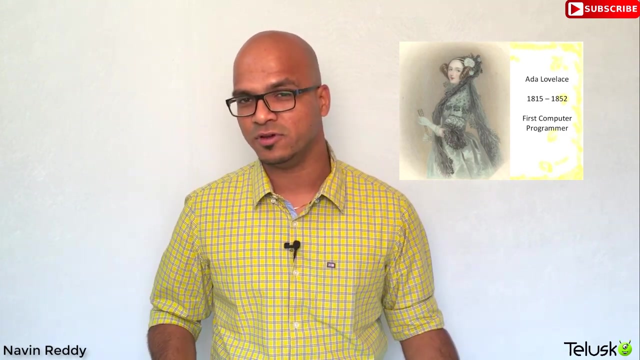 But then this generation. we talk about devices which are computers, right? So in 1822, Charles Babbage came up with a concept of mechanical computer And with him there was a lady called as Lady Ada Lowlands. She created the first programming language. Everything was awesome. Everyone thought. you know that will change everything in future. 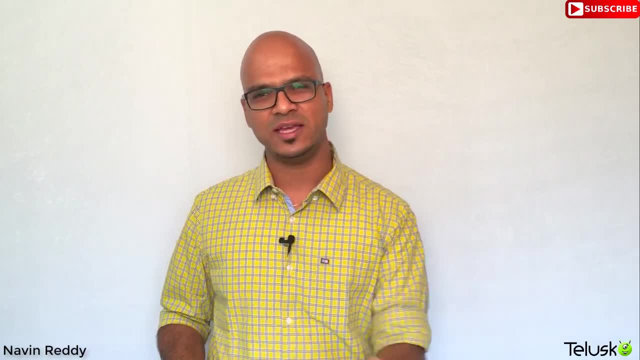 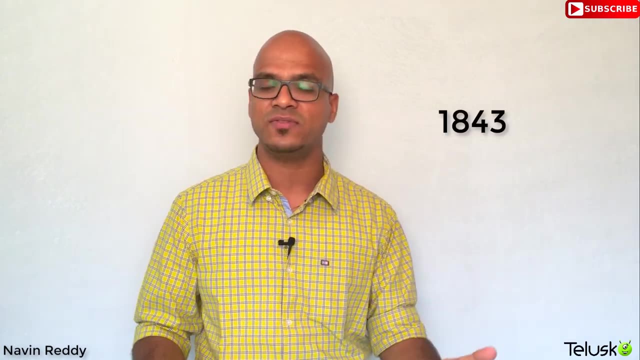 But then the problem is: for next 70 years there were not any language. I mean, can you imagine that We got the first language in 1843, I guess, And then after that we got the second language, The second language around, in second, I guess, Second World War or maybe after that? 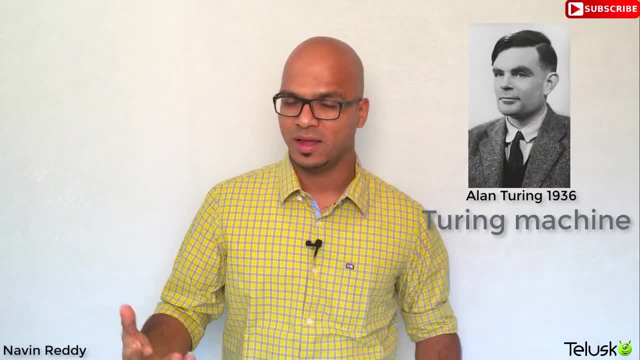 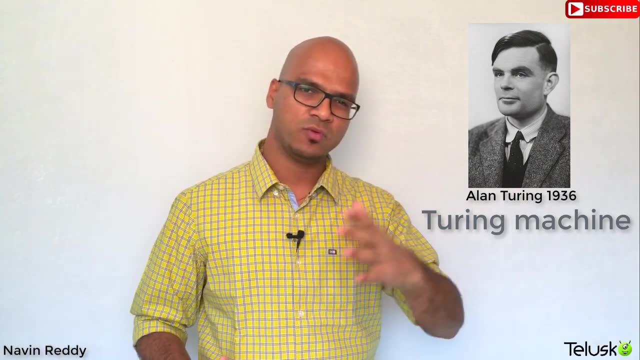 In fact, you might have heard about Alan Turing During Second World War. Alan Turing came up with the concept of Turing machine Because, you know, in Second World War they wanted to decrypt the message And to decrypt the message. it was mathematician's job to decrypt the message. 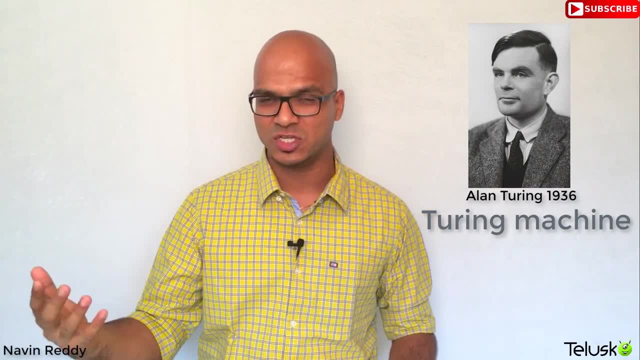 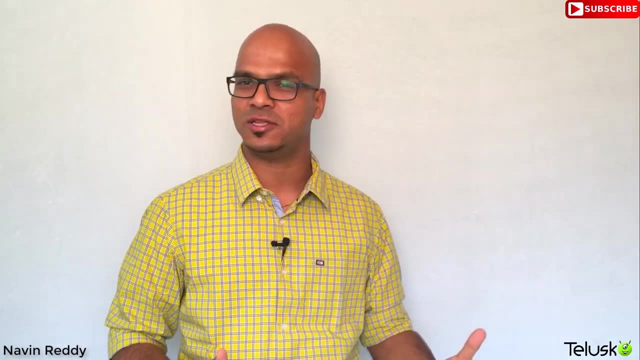 And then, you know, it was very difficult for them to decrypt a message by people, And that's why he came up with the concept of computer. Let's create a computer who will decrypt the message. That was Turing machine And in fact at that time it was awesome. 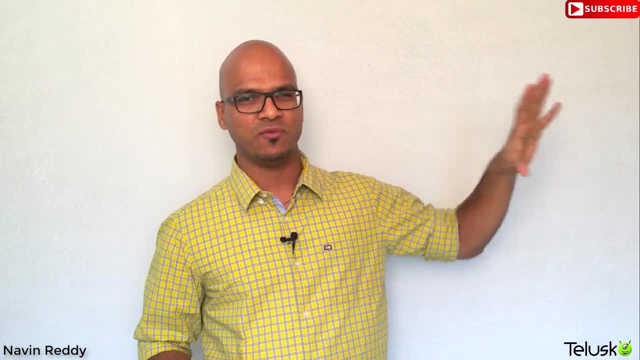 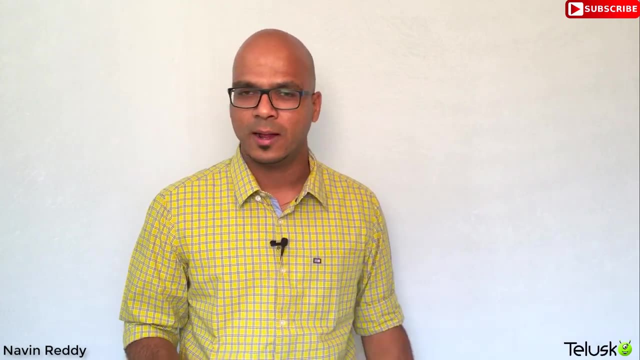 And then you know people thought, okay, that's what computer will be. A computer will be a machine in which you have to give the input and it will process your data and it will give the output. But then they wanted some way to interact with the machine. 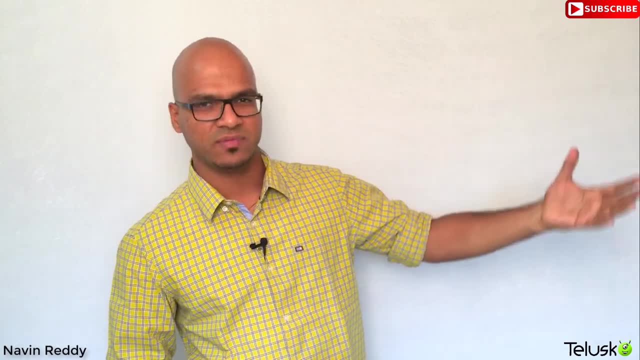 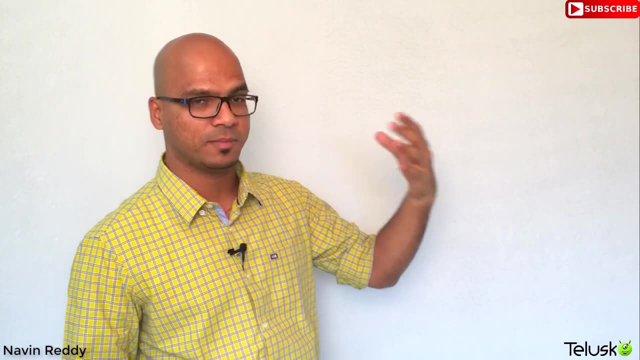 And they came with the concept of electronic machine. Instead of going for the mechanical devices, they came with the concept of electronic machine And maybe in 1940s or late 1940s they came with the concept of electronic machine, Where it will be having vacuum tubes. 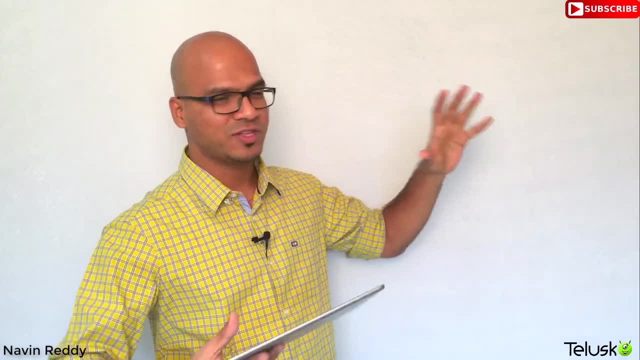 Right, Can you imagine vacuum tubes? I don't know what the size of vacuum tube, But then it was a very big machine. In fact the first computer was so small. I mean, can you imagine So small? It was so small. 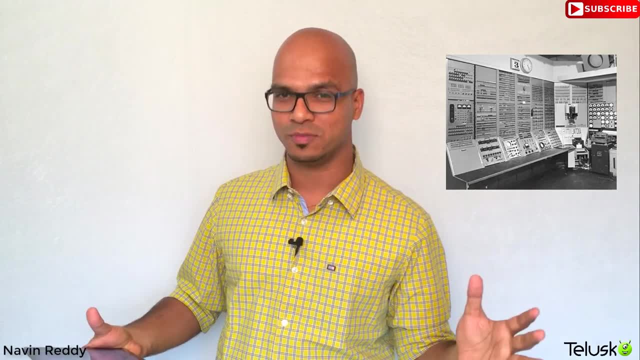 It used to take only four rooms. There is one room- It used to take four rooms- just to accommodate that one computer. Huge, right, Not small. So it was a very big machine And it was working with a vacuum tube. 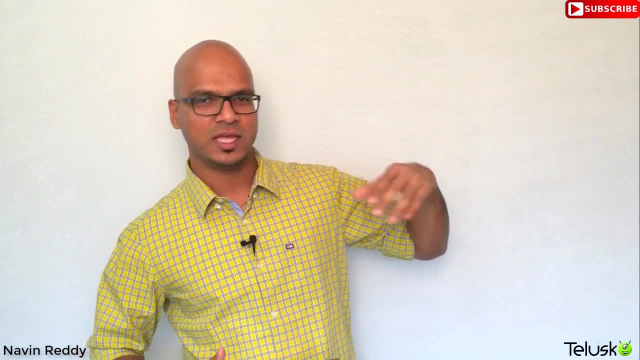 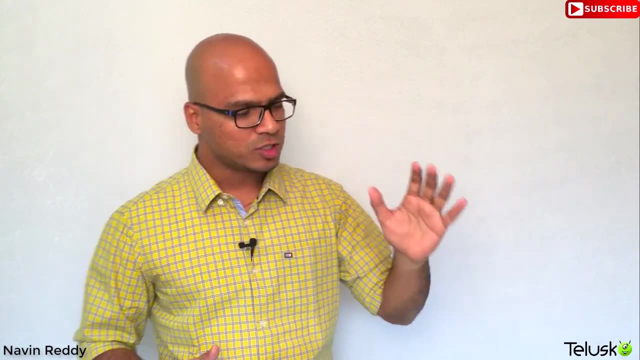 So they thought about: let's reduce the size of it. Instead of going for vacuum tubes, they went for semiconductor, They went for semiconductors, They went for transistors- Right. And then they also thought about: let's create a CPU. 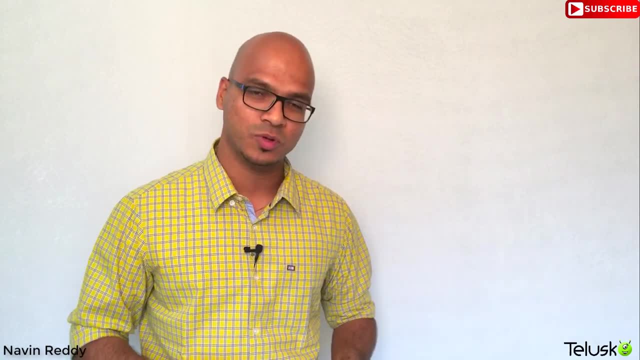 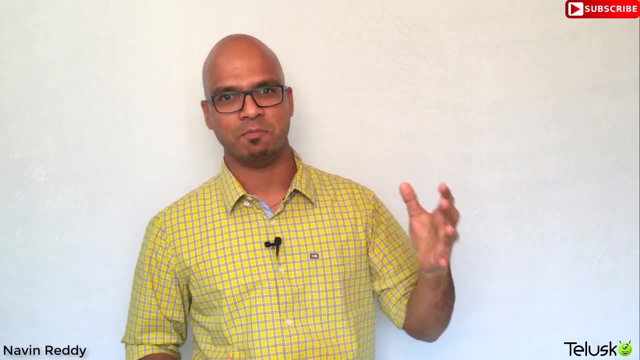 Because you can program CPU Right. You can ask CPU to do things for you. Now what happens? You know, we always say computers are intelligent devices. They are smart. I mean, do you think computers are intelligent than humans? Not exactly. 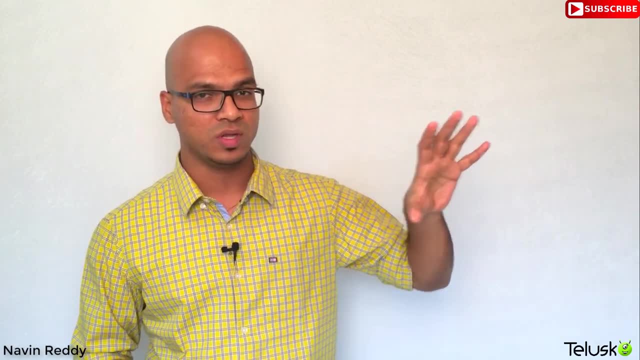 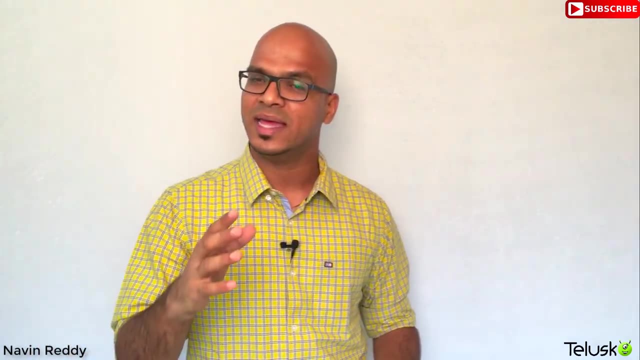 Computers are not intelligent than humans Because computer can do only those things which human say human ask computer to do. Right, How can you talk to computer? Is it easy to talk to computer? Yes, If you can use a common language, which I mean a computer and human can understand. 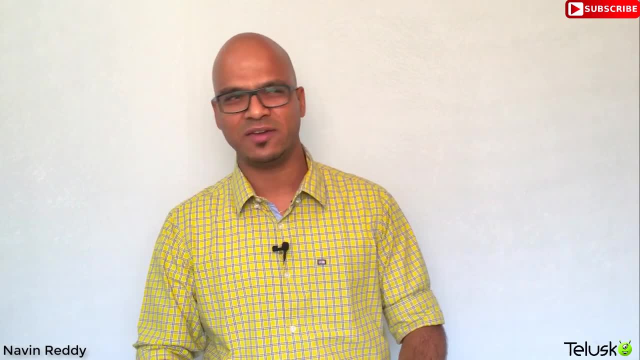 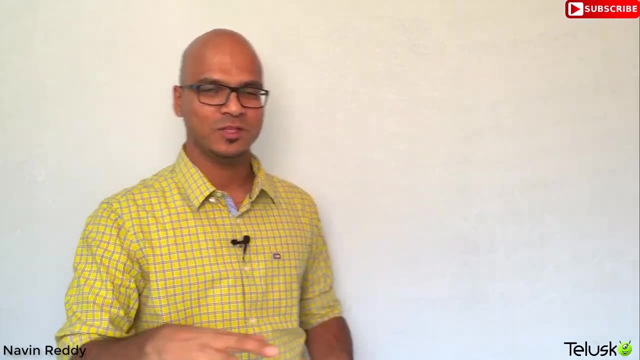 Right, And that's why they came up with the concept of machine language. So what is machine language now? It's a language which works with 0 and 1, which is binary language, Right? So just imagine if you want to talk to a computer using 0s and 1s. 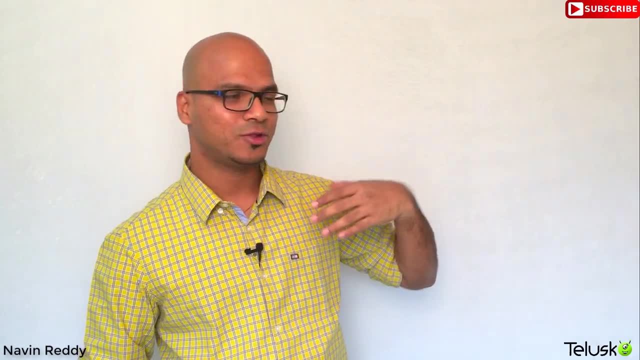 That will not be a good way. Just imagine: you know you have a computer with you And then you are talking to computer. hey, 101, 001.. The thing is: computer will understand, But a computer gives you a response. 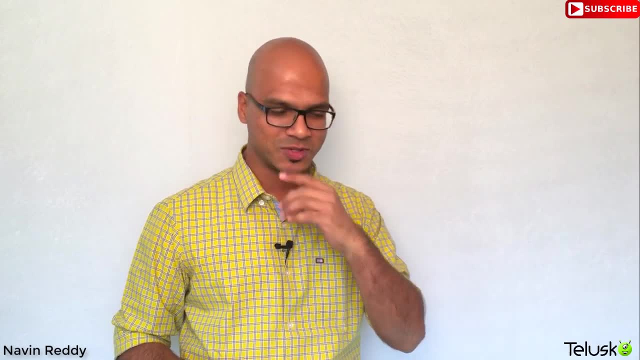 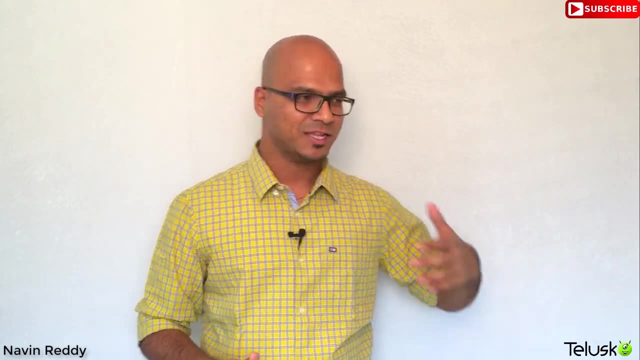 That will be difficult to decrypt, Right? So that's the issue. The second thing is: let's imagine if you are talking to someone on Facebook using 121 and 000.. I mean, just imagine if you are saying 121, 000, then you will be getting some bad words. 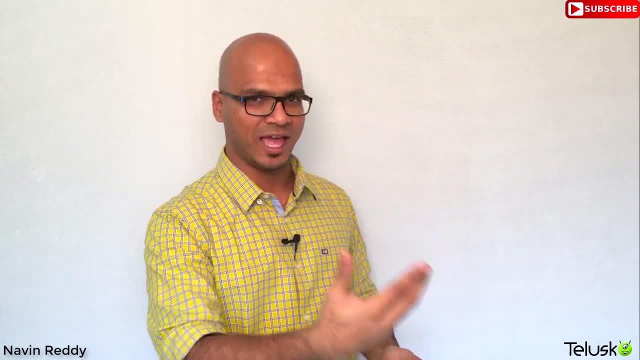 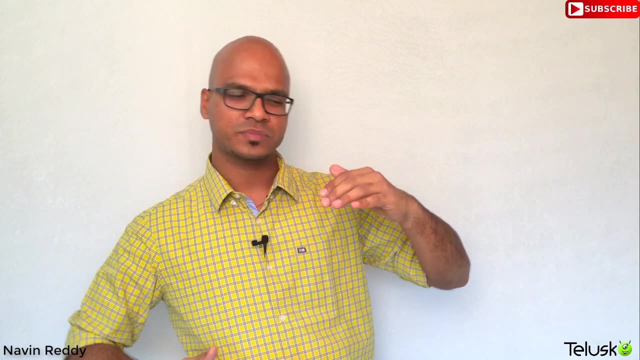 from the other side, So you have to make sure that you don't use those language with humans, And that was difficult for humans to work with that language. So we wanted a language using which, actually, that language should be somewhere similar to English. 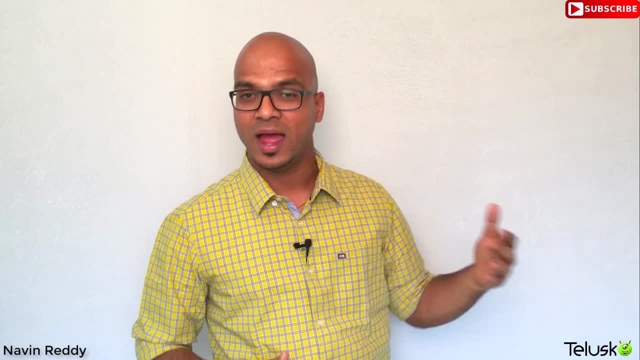 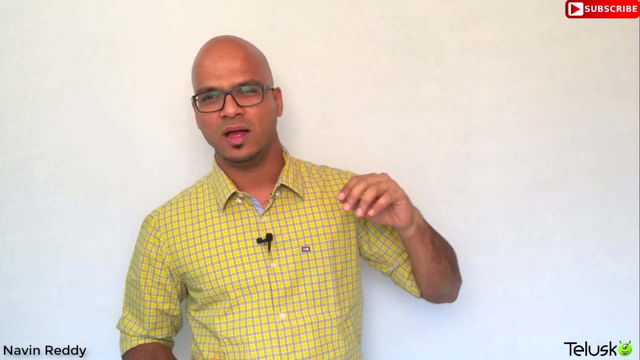 And then it should be also understandable by computer also. And that's where they came with the concept of assembly language. Now, assembly language was low-level language. Now, when you say low-level language, it means your computer CPU can understand that. what? 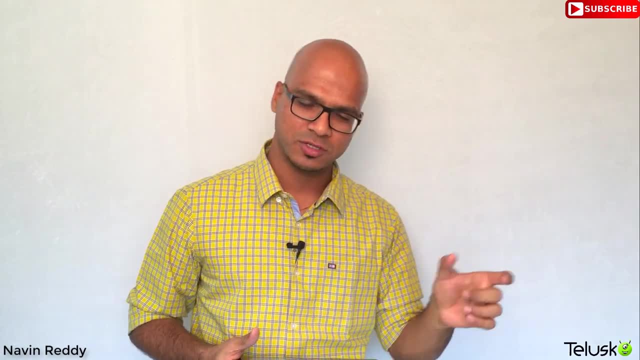 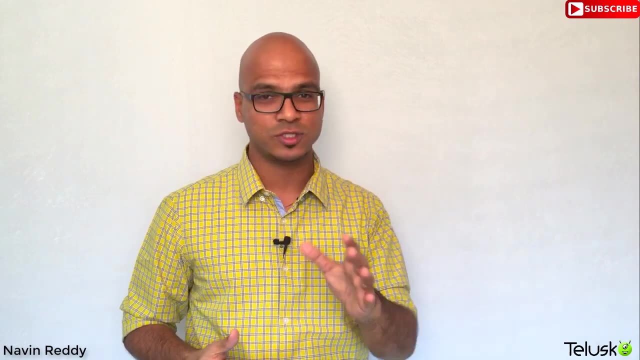 exactly that. language means There will be only an interpretation, So you just have to write the code and your CPU will understand what you are saying. That was assembly language And it was awesome. Now the thing is, assembly is a low-level language not structured properly. It was having lots of problems creating big softwares. In fact, initially it was good to work with normal CPUs, But now we are living in a generation where you have octa-core CPUs, where you will be having huge amount of data to work with. 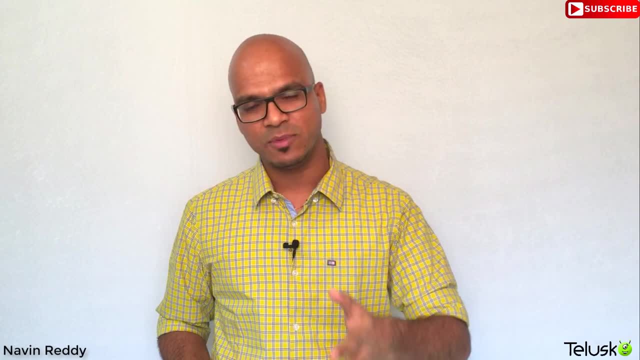 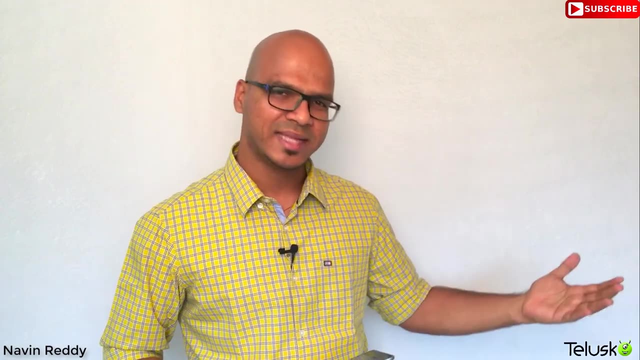 So assembly is not that efficient in that case And that's why we came with the concept of high-level languages. Now, when I say high-level languages, there were lots of languages at that time, Mostly at that time. when you say computers, they used to only use for scientific purpose. 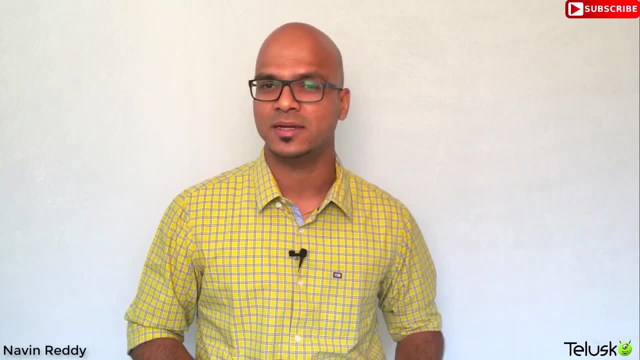 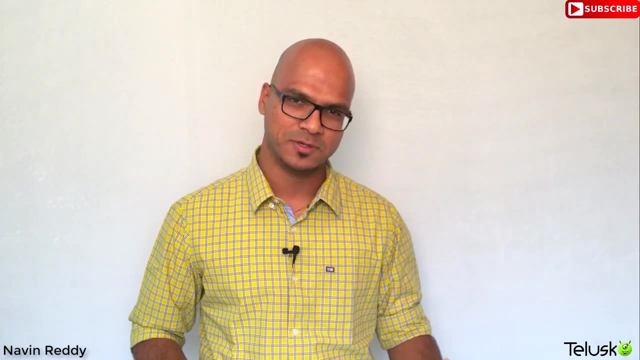 research purpose. Maybe mathematician will used to use that, Maybe for rocket launching- I don't know at that time if they were launching it, But then they were using these computers only for that purpose. So they wanted a language using which they can actually work with maths. 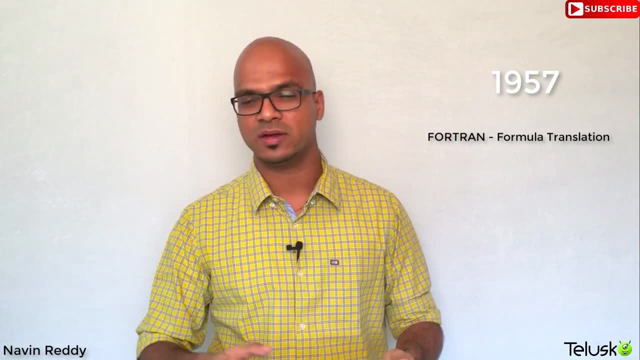 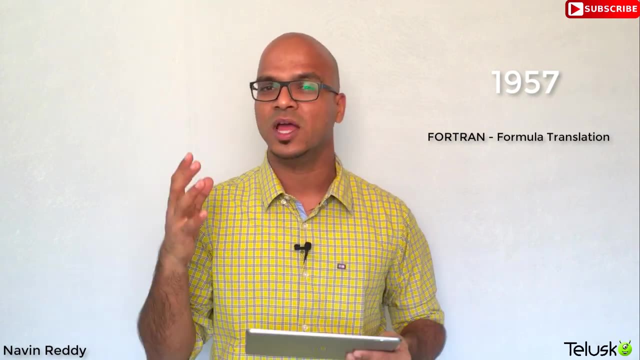 And they came with the concept of Fortran, And Fortran came in year 1957.. Now, if you don't know the full form of Fortran, it's very easy: It's formula translation. That means you can convert your mathematical codes into programming codes. 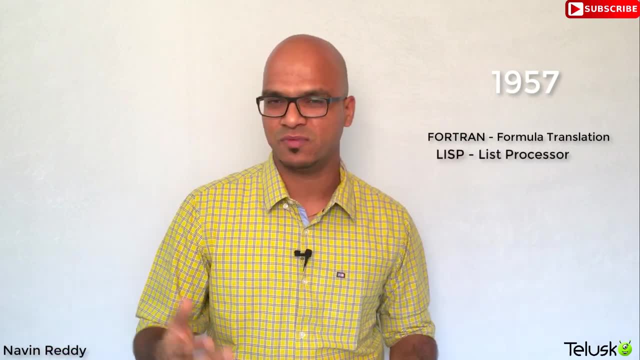 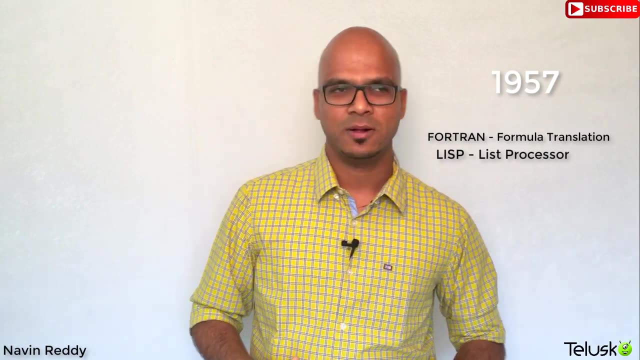 Everything was good. Then they also came with the concept of LISP, which is leased processor. That's weird LISP, L-I-S-P, And it was also used for maths, But then all the languages are made for maths, right. 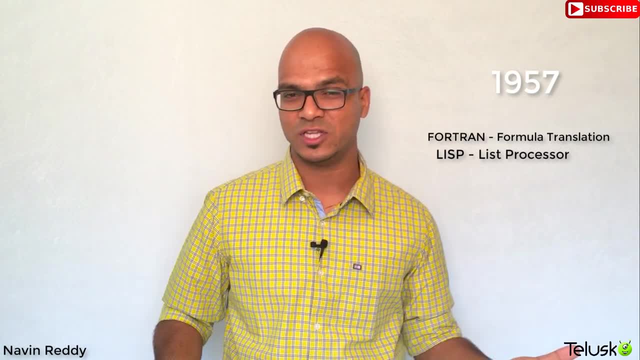 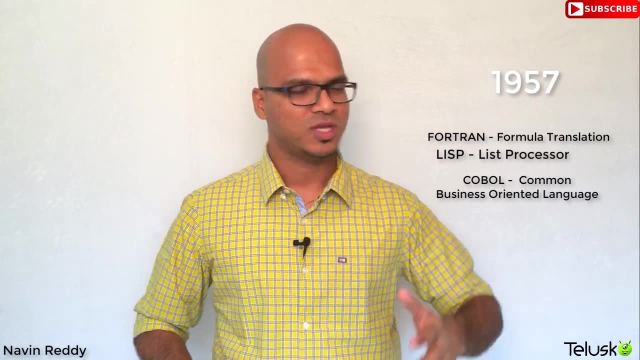 What about business? Because we also want a language to work with business. right, And they came with the concept of COBOL. Now COBOL stands for Common Business Oriented Language. So everything was good. We got Fortran. 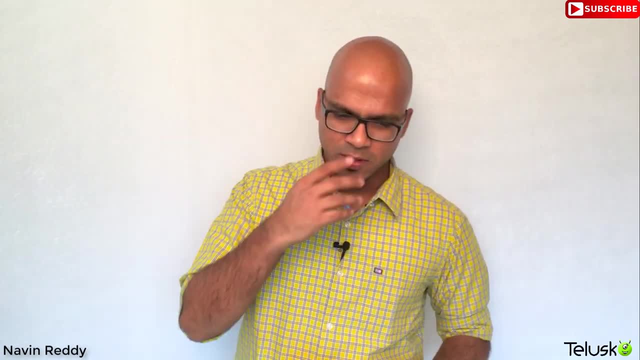 We got LISP, We got COBOL. But then you know, let's say, we got all these languages now And you want to teach. In fact, after this also, they got lots of languages. We got B language. 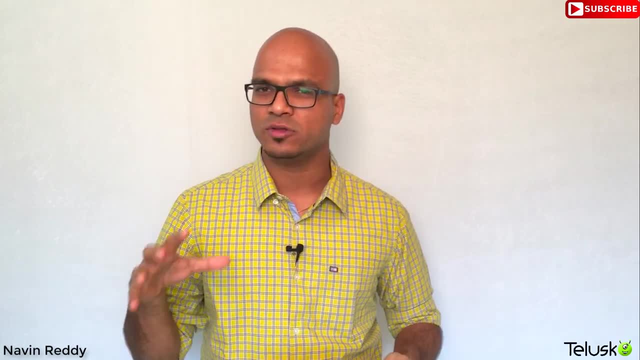 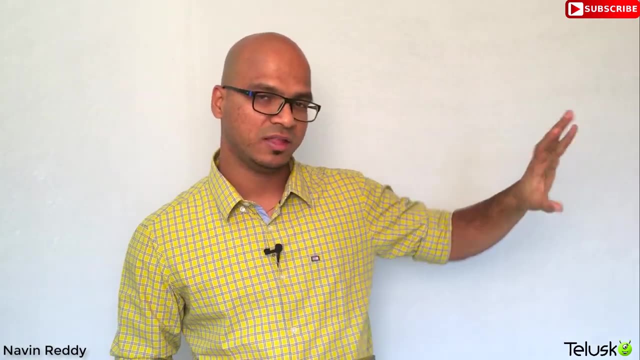 We got BCPL. But then let's say, if I am a teacher, if I want to teach a programming language to a person, it was very difficult to teach all these languages because there were different languages and different perspective, right. So we wanted our language, using which you can actually teach programming to people. 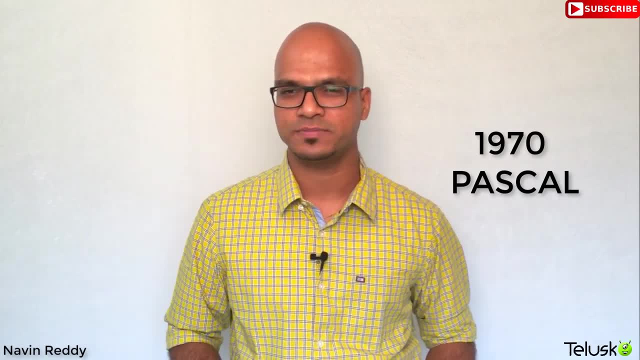 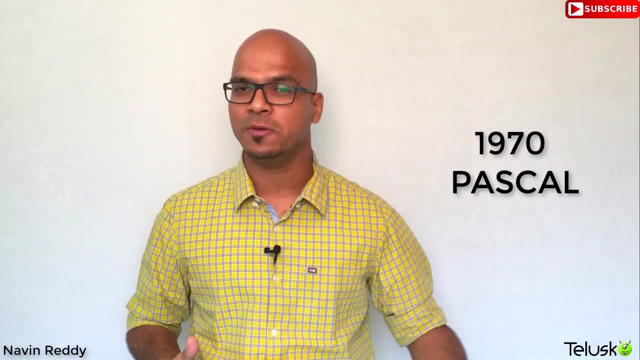 And that's where Pascal came into picture. So in 1970, we got a language called as Pascal- Now Pascal. using Pascal, you can teach to people, And then later it was also implemented for business purpose. You can actually use Pascal to make softwares. 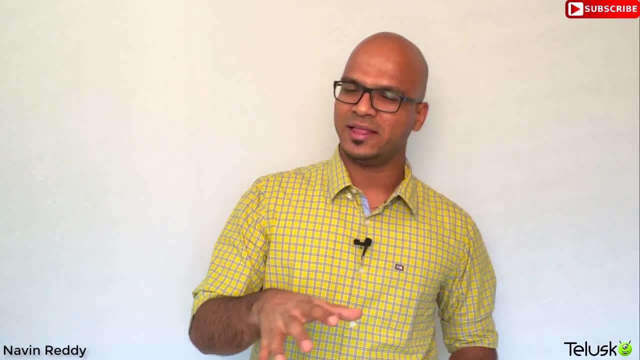 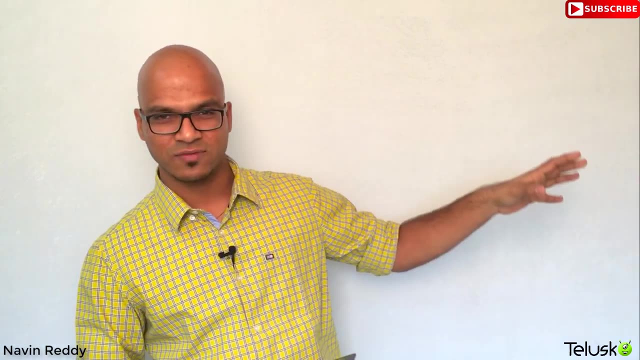 And everything was good. We got Pascal. Then in late 1970s or maybe late 1960s- at that time there was a guy called as Ken Thompson And then he thought: you know, we have lots of languages. 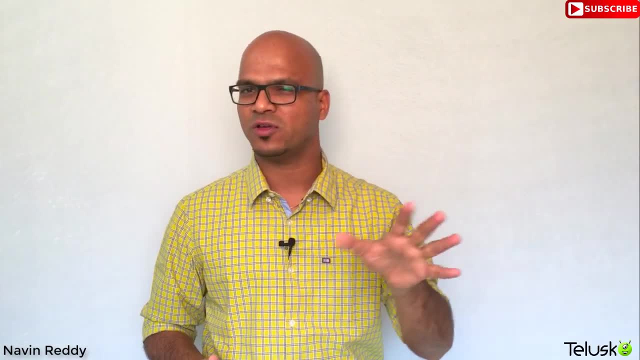 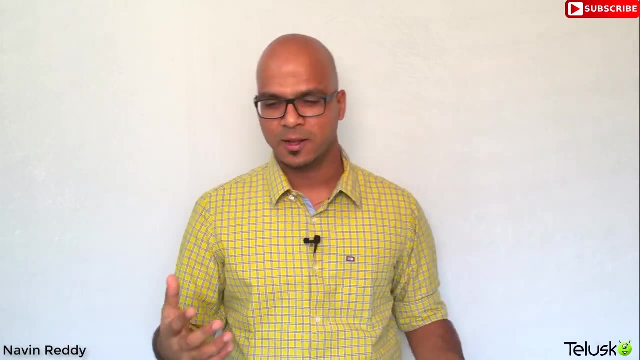 In fact, Ken Thompson at that time also created one more language called as B language. I don't know if you have heard about that. We also have a B language Now. B language was there and everyone was happy. We got all these languages. 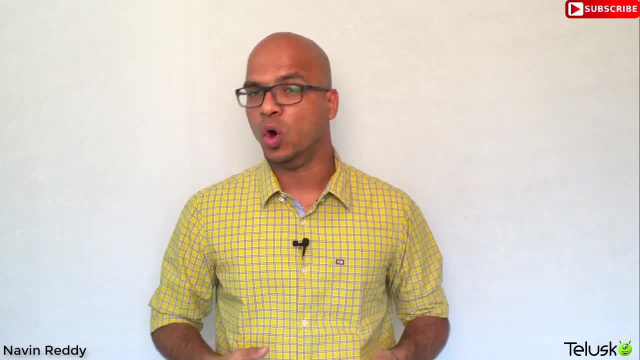 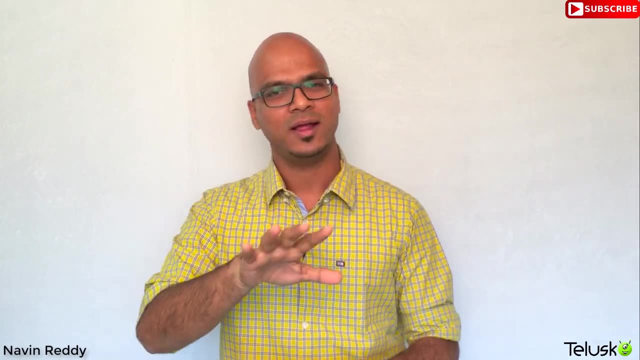 But then, if you heard about this, we also had one more OS at that time, OS which is called as UNIX U-N-I-C-S. And I know you are talking about UNIX, right? No, The earlier one was U-N-I-C-S. 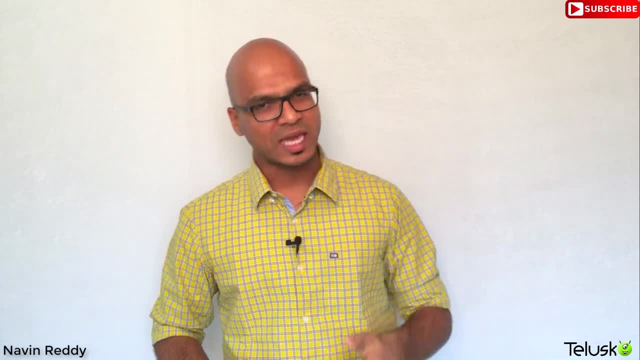 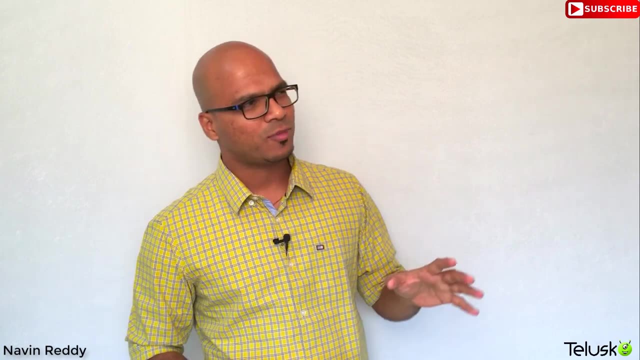 And then it was made in assembly language. So Ken Thompson wanted to redesign that OS using- what do you say? a modern language. So he thought about: can we use Pascal? Can we use B language? No, Can we use some other language? 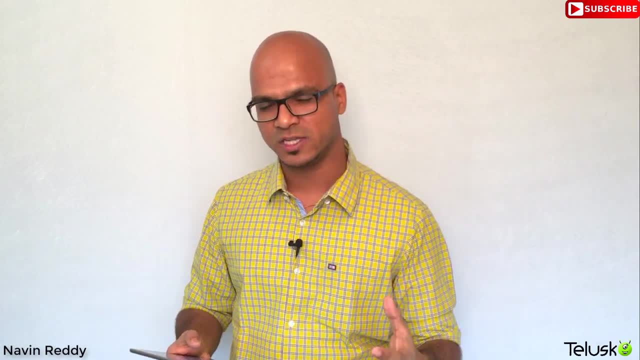 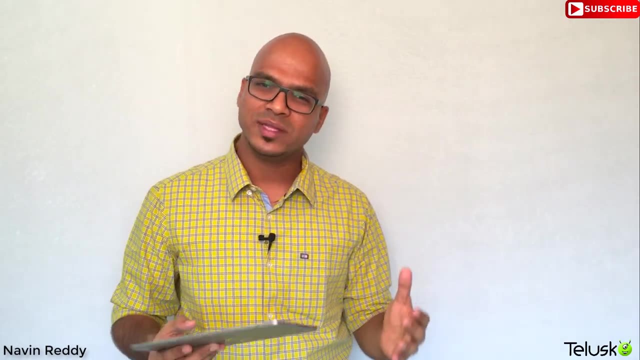 And then he thought about: let's create a complete language, Because see, all these languages have their own language, They have their own way of working, right? I mean, they were used for a specific reason, So he wanted a language which will be complete language. 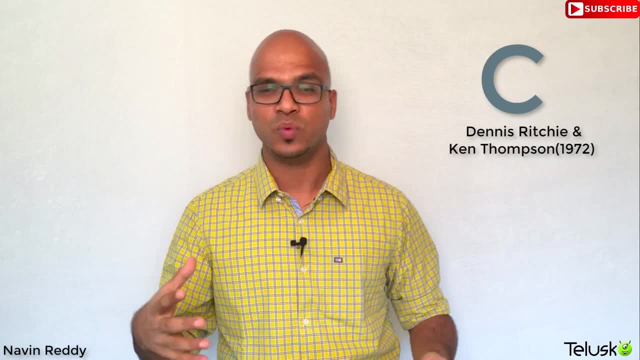 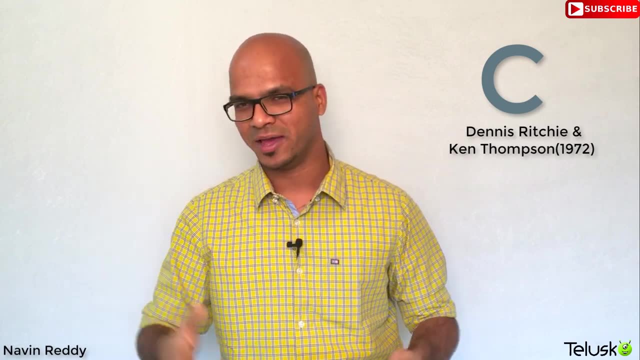 And that's where they came with the concept of C language. Now Ken Thompson, with Dennis Ritchie they came with the concept of C programming, And again it was made in Bell Laboratories. Now you might have heard about that lab right. 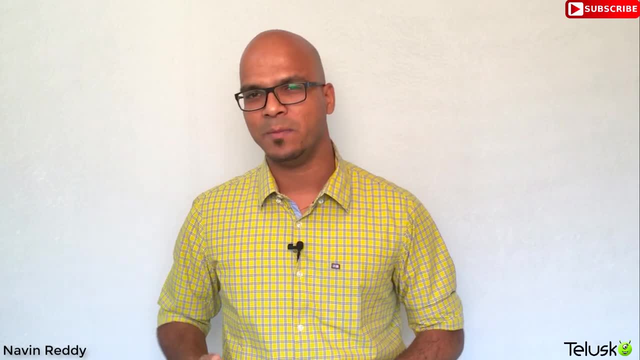 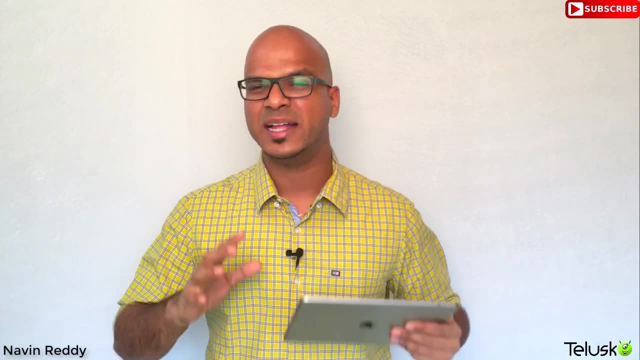 So we have all these languages like C++, C, made in Bell Labs, So we got C. Everyone was happy. In fact, C is also called as mother of all the languages Because it is the first complete language. You can do anything you want. 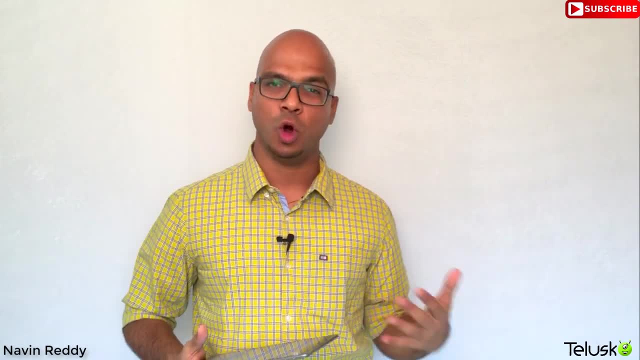 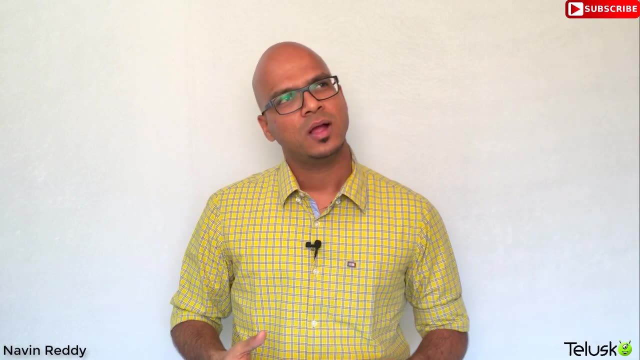 You can build networking services, You can build OS, You can build embedded software, You can do everything using C language. But then there's a trick here. The trick is what if see in real life we work with objects right? 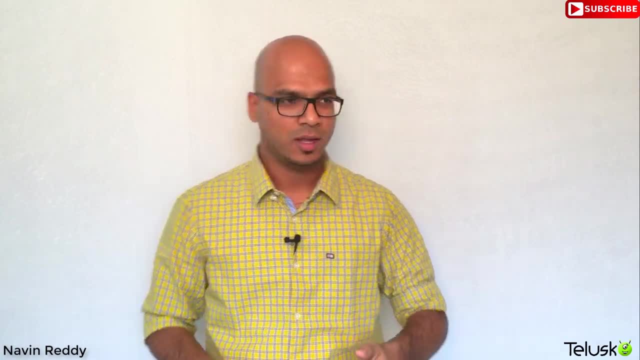 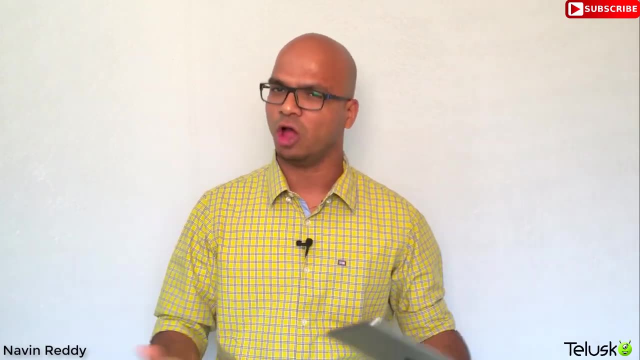 In fact, the thing which I'm holding here, it's an object. The thing which is behind me, it's an object. The thing which is shooting me here is an object. right, In fact, these things around me, those are objects. 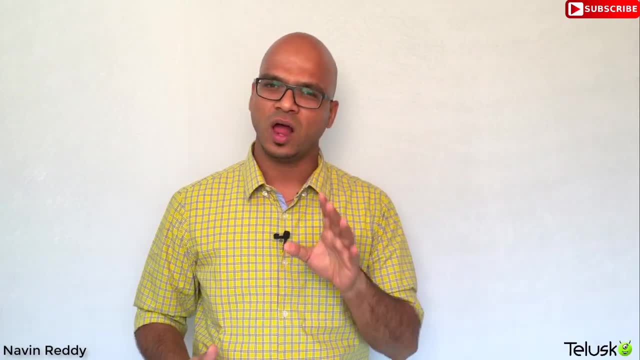 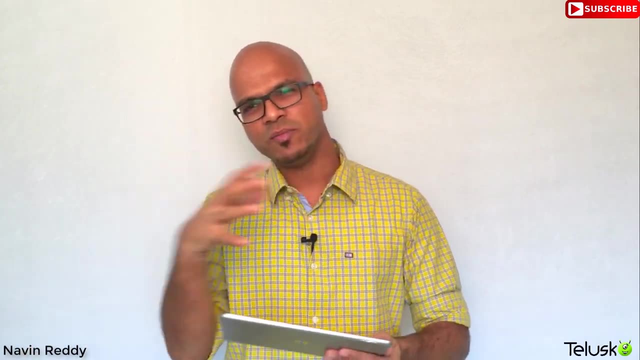 But in virtual world, which is your programming world, we are working with C language. So everything is good. We got C, We got object concept. How can we merge this? Because in real life we use objects. In virtual world, which is programming world, we use procedures.